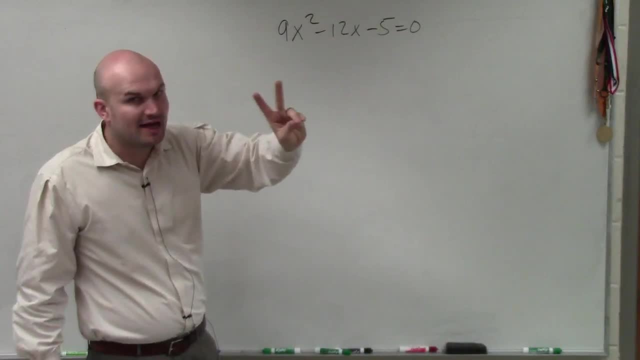 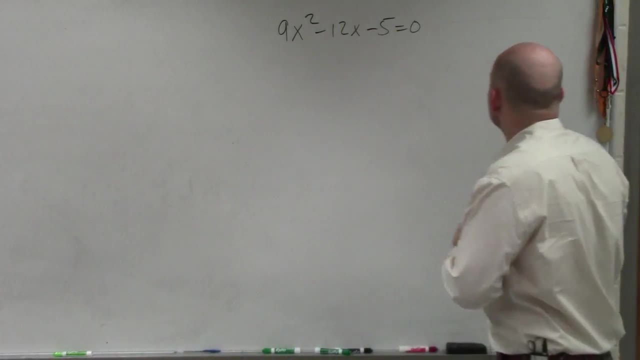 out. we want to be able to rewrite our middle term as two separate values And, rather than filling them in a box, we're going to factor by grouping, which we actually talked about before in this class. But either way, the first thing we need to do is do A times C. 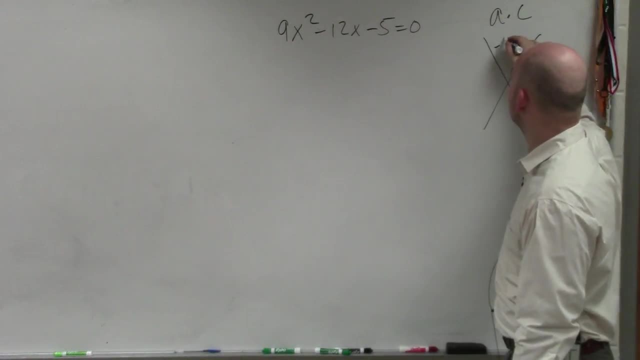 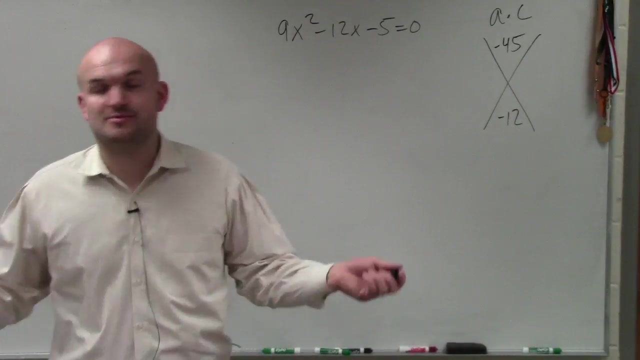 A times C, Nine times negative five is negative 45. And then the add to give us negative 12.. Now I get a lot of students that get stuck and they say, Mr McGlung, I don't know, you know what to do, you know? next, The most important thing that I would say: guys even. 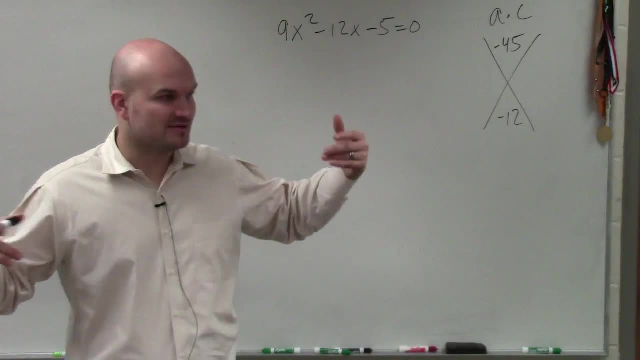 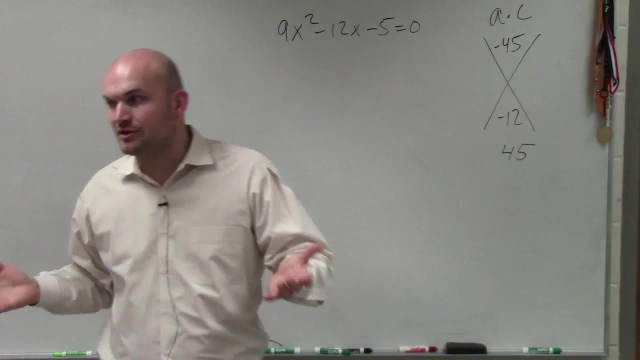 if you get stuck, all right. even if you can't figure it out on your test, write down all of the factors of 45. All right, And this isn't that difficult. The way that I want you to do it is: 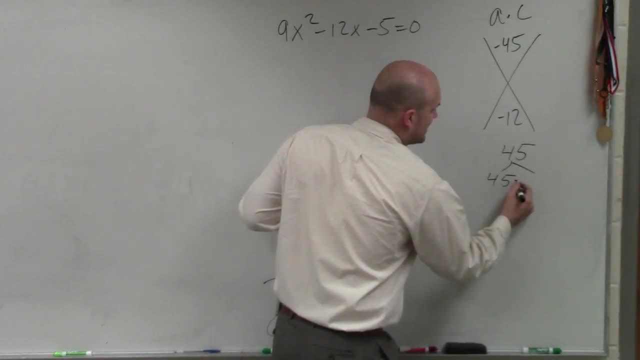 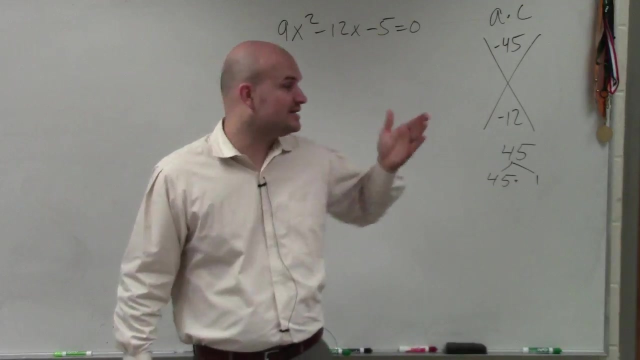 Okay, Hold on a minute. Before we start over off topic, let me just show you part two first. OK, econometrics, let's say So. it's a set of numbers, Let's see. Okay, so it says best start. then you can always do it with 45 is 45,, which obviously 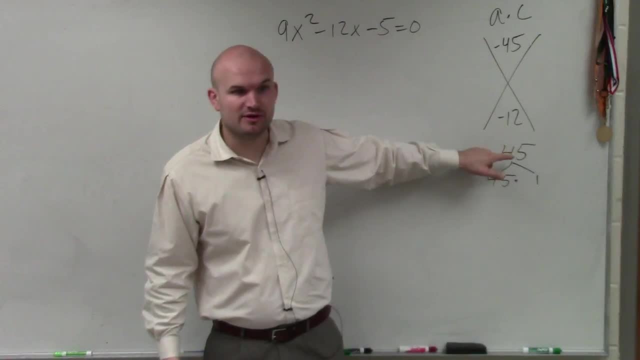 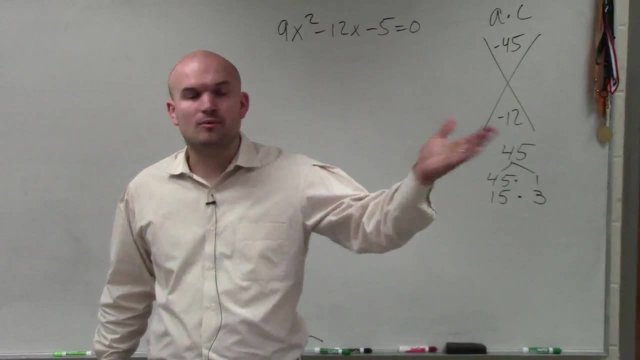 let me see. obviously you can always start with 45 x 1. Then just start working with numbers to go from one. Now let's say two Is two divisible into 45? No, it's not right. So then we go to three. 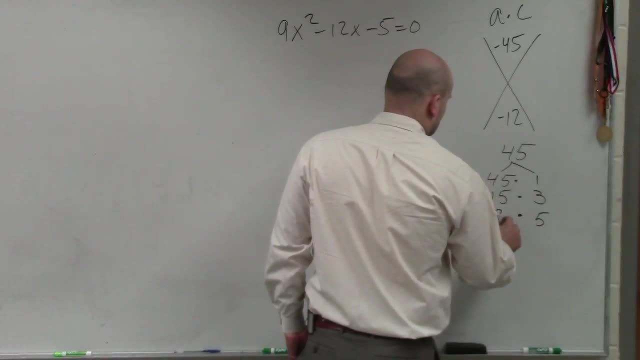 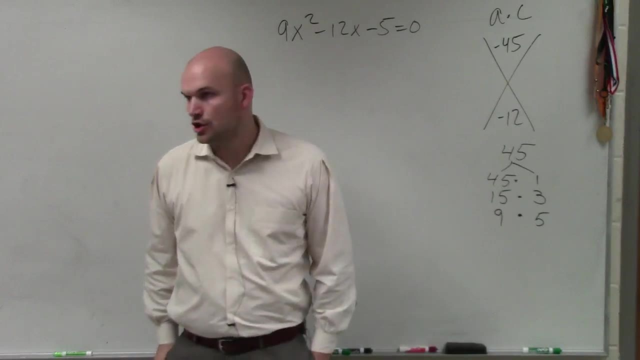 45. Yes, And then we go up to 6.. Is 6 divisible into 45? No, 7? No, 8? No, And then I get back up to 9, which I already know is divisible. so therefore, I'm all done. So these are the 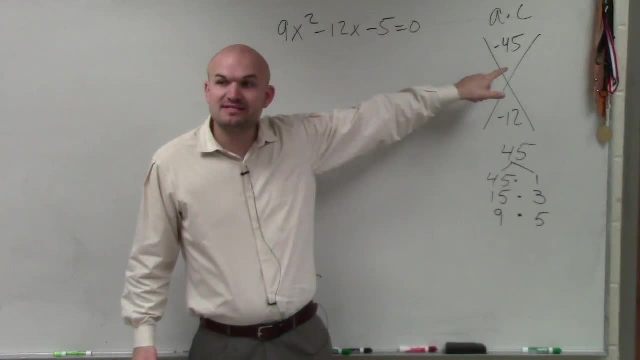 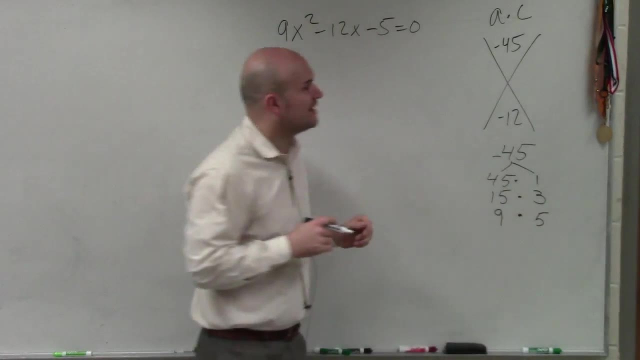 only factors. Now we are multiplying to give us negative 45.. So just think, listen to my mind, my thought process: It has to multiply to give you negative 45 and add to give you negative. If you're adding a positive and a negative number and your answer is negative. 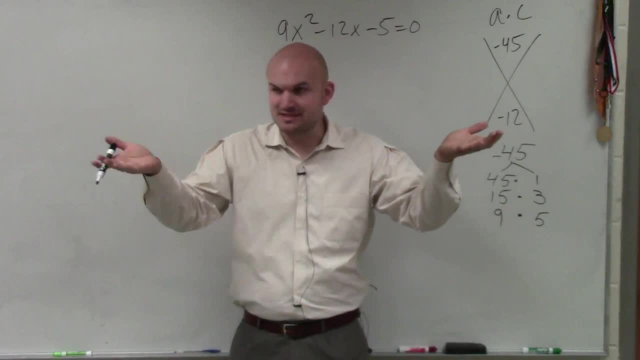 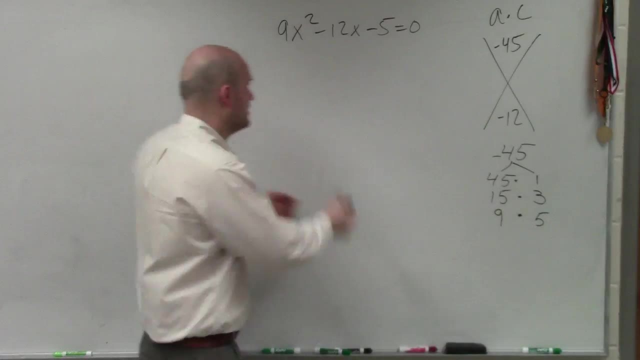 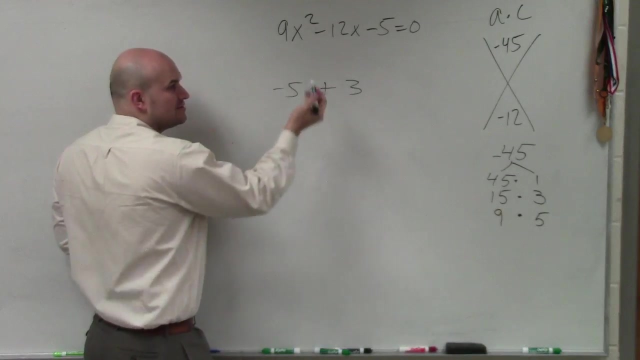 should the negative or the positive number be larger? in absolute value, The negative number should be larger, Think about it. Negative 5 plus 3.. In absolute value, which one is larger, The 5 or the 3?? The 5, right. So a larger negative 5, absolute value of it plus. 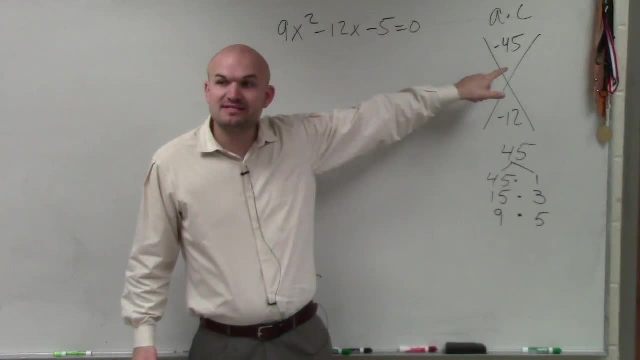 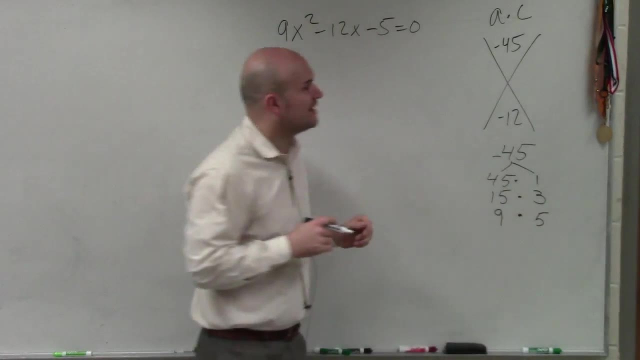 only factors. Now we are multiplying to give us negative 45.. So just think, listen to my mind, my thought process: It has to multiply to give you negative 45 and add to give you negative. If you're adding a positive and a negative number and your answer is negative. 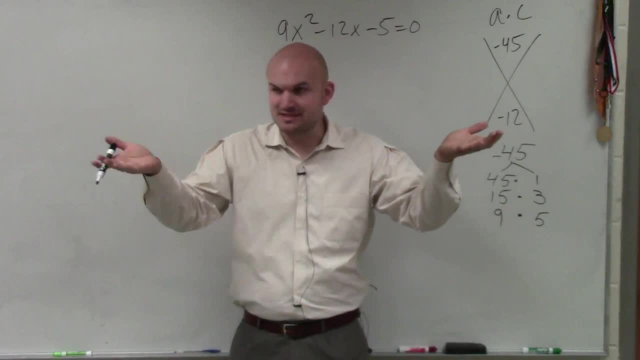 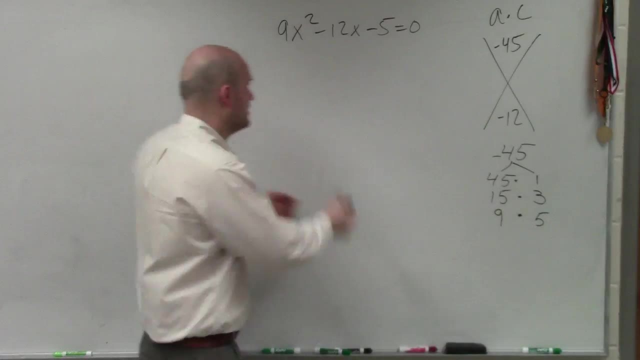 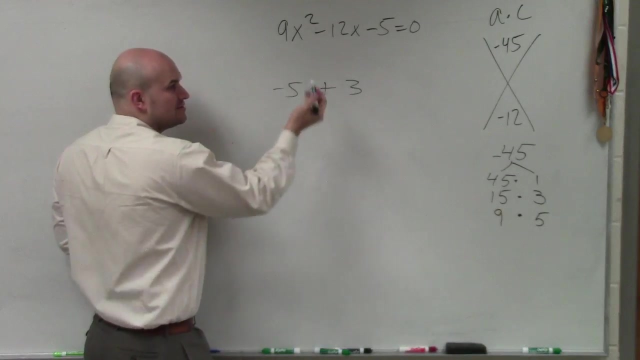 should the negative or the positive number be larger? in absolute value, The negative number should be larger, Think about it. Negative 5 plus 3.. In absolute value, which one is larger, The 5 or the 3?? The 5, right. So a larger negative 5, absolute value of it plus. 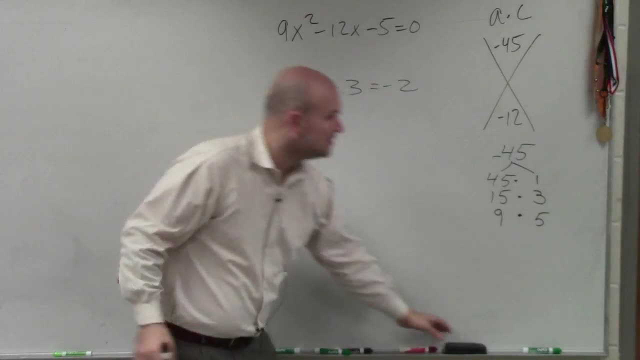 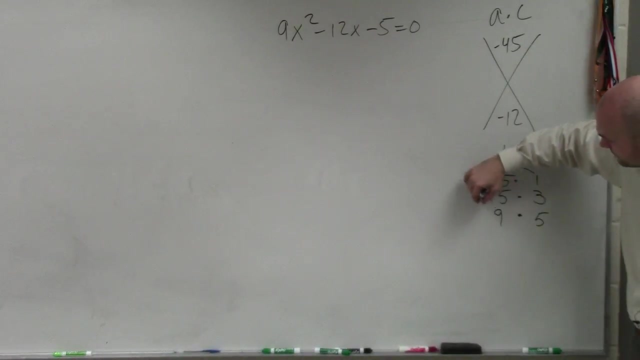 3 is going to equal negative 2, right, It's going to give you a negative number. So there means I have to multiply And therefore, since I'm adding these two factors and my sum is negative, then my larger factor has to be negative. And now, when I look at this, 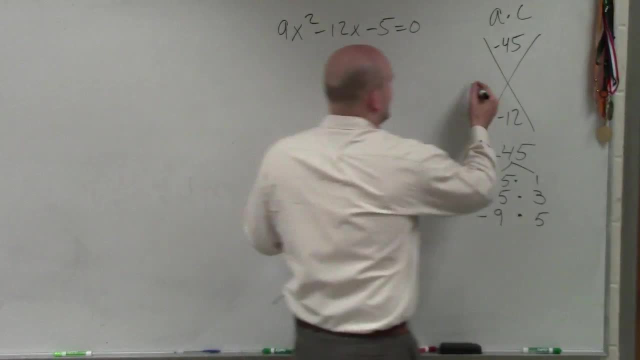 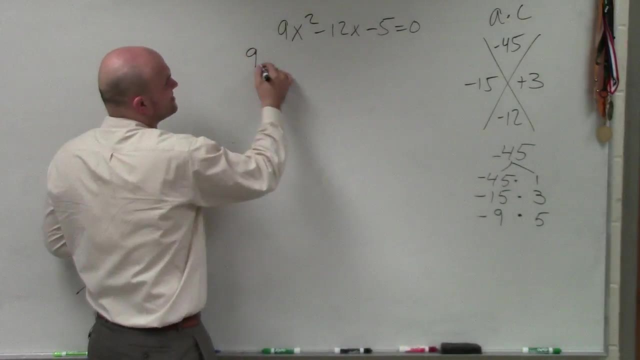 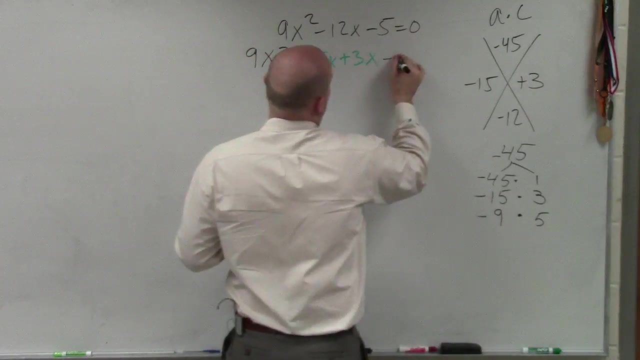 actually, which of these add up to give me negative 12? Negative 15 and positive 3.. Now I'm going to do just like what I did last time, but I'm not going to fill it into a box. I'm going to say 9x squared, And then I'm going to say minus 15x, plus 3x, minus 5,. 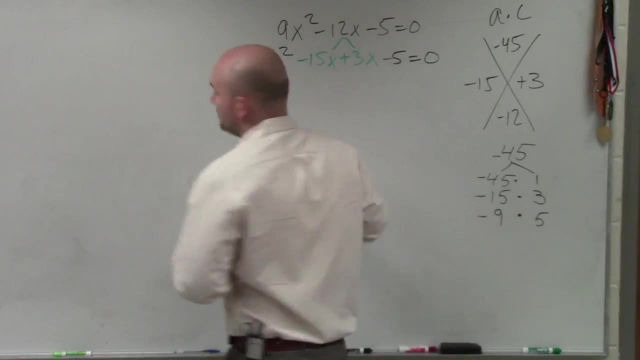 5 equals 0.. Does everybody see what I did? I just rewrote the equation. That's all I did. I didn't change it or do anything else with it. I didn't put it in a box, I just rewrote it. 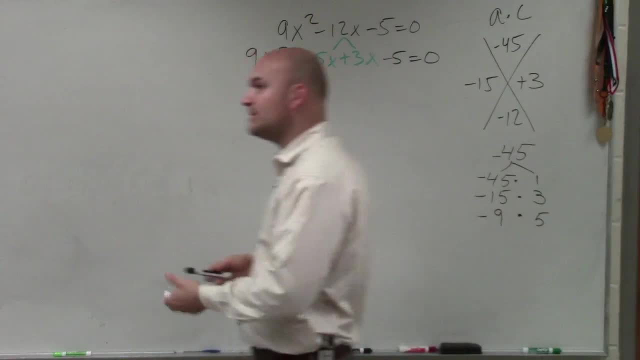 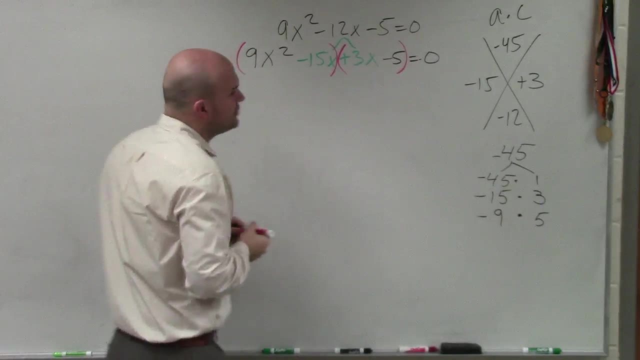 But I mean, I showed you guys how to rewrite this last time And now what we can do is a factoring technique, which we call grouping, where you group the first two terms and you group the last two terms, And basically what we have already done in this class is: we talked about grouping. 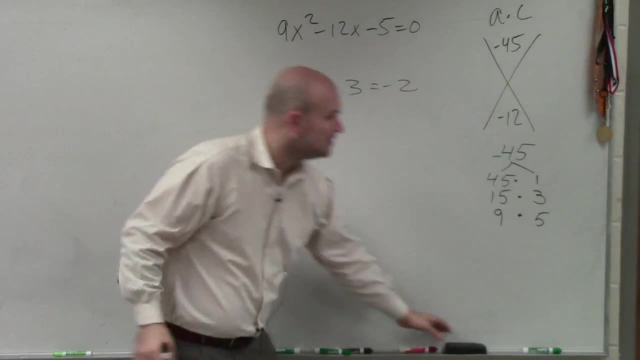 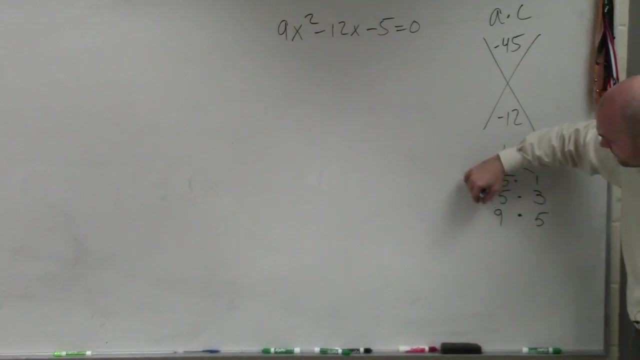 3 is going to equal negative 2, right, It's going to give you a negative number. So there are two factors, two factors. So since I'm adding these two factors and my the sum is negative, then my larger factor has to be negative. And now, when I look at this, Ashley, 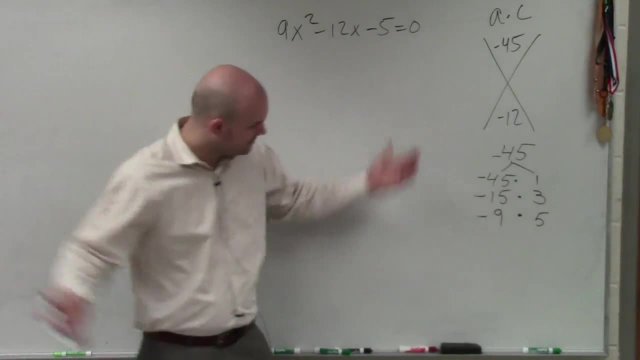 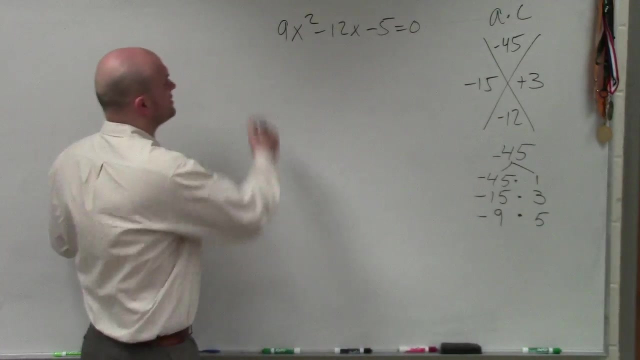 which of these add up to give me negative 12? Negative 15 and positive 3.. Now I'm going to do just like what I did last time, but I'm not going to fill it into a box. I'm going to say 9X squared, and then I'm going to say minus 15X plus 3X, minus 5.. There you go, There's. a cost Model, by the way, And when I look at it and I notice that I have a minus 15.. There's a negative 12 right there, And then again I multiply 2.. So I take that and I multiply this, multiply that and I multiply the other half, And what are we doing? Well, we're multiplying. 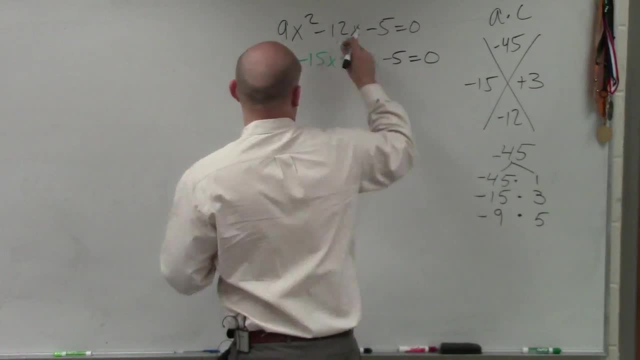 5 minus 5 equals 0.. Does everybody see what I did? I just rewrote the equation. That's all I did. I didn't change it or do anything else with it. I didn't put it in a box, I just rewrote it. 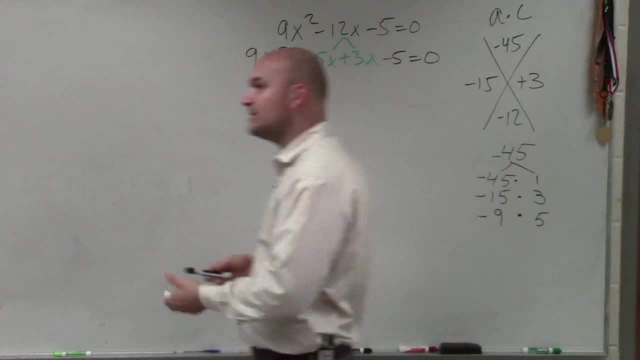 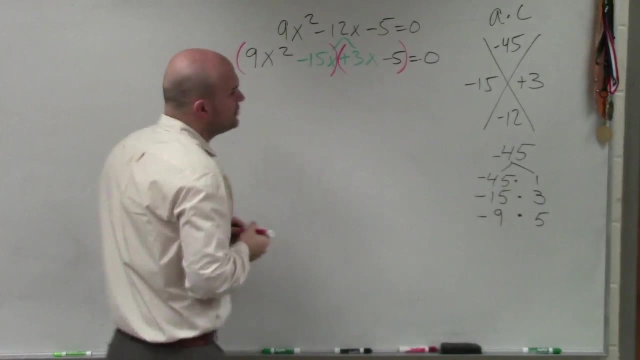 But I mean, I showed you guys how to rewrite this last time And now what we can do is a factoring technique, which we call grouping, where you group the first two terms and you group the last two terms, And basically what we have already done in this class is: we talked about grouping, but 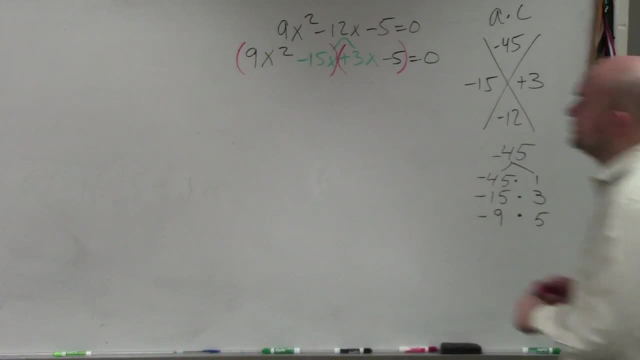 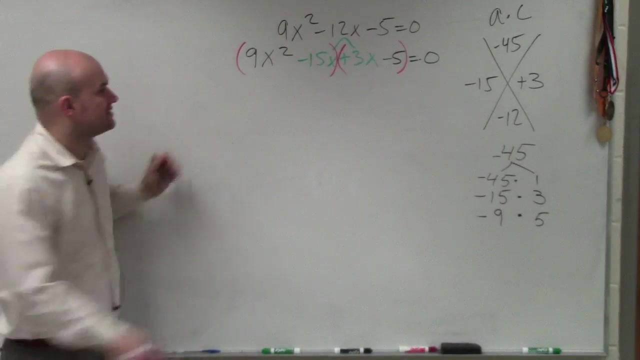 we also talked about factoring out the GCF. Now, all you're simply going to do is factor the GCF out of each of these expressions. So we look at the first two and say: what do these have in common? What is my common factor? 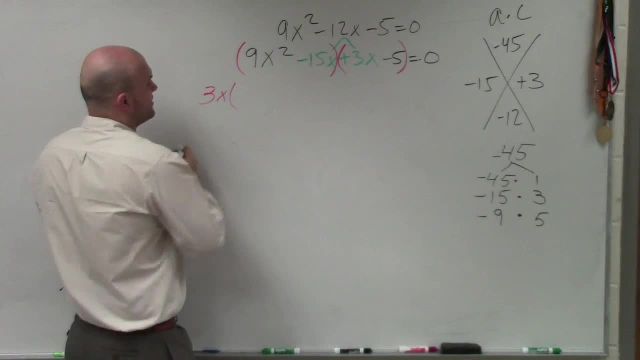 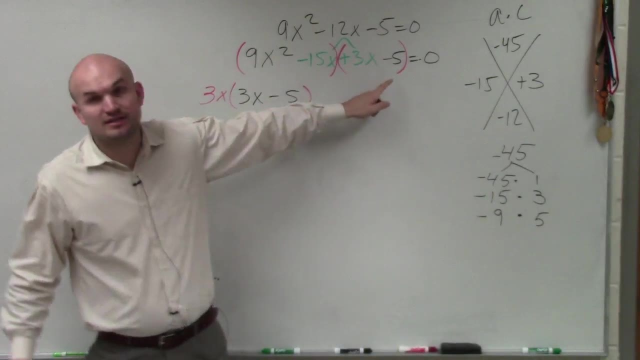 You could say a 3x, And when you factor out a 3x, you're left with 3x minus 5.. Then I look over here and I say, is there anything I can factor out of these? No, So therefore I can factor out a positive 1.. 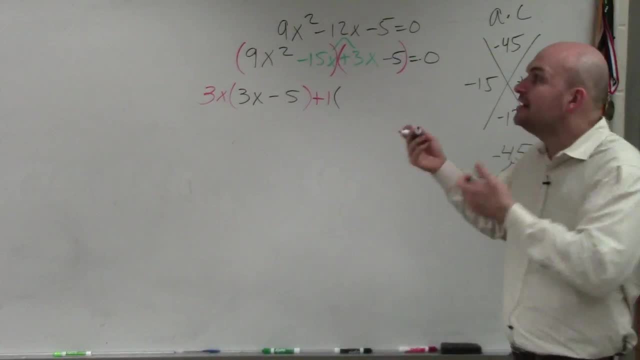 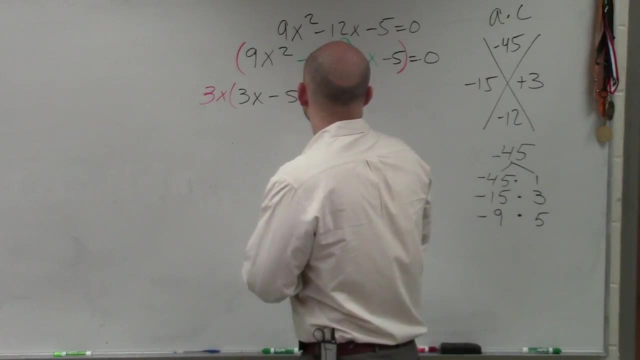 You're always going to have to factor out something, And if they don't have anything in common, Then factor out a positive or a negative 1.. OK, Tyler, And then therefore, we're left with 3x minus 5.. 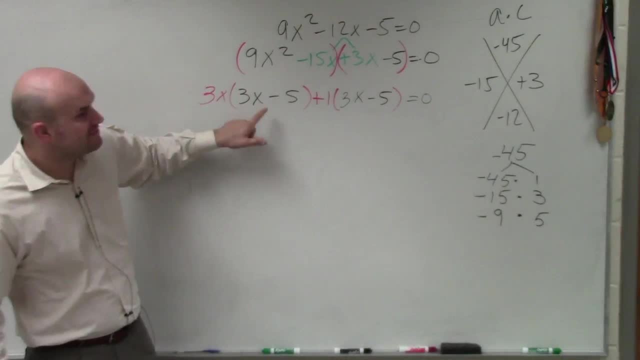 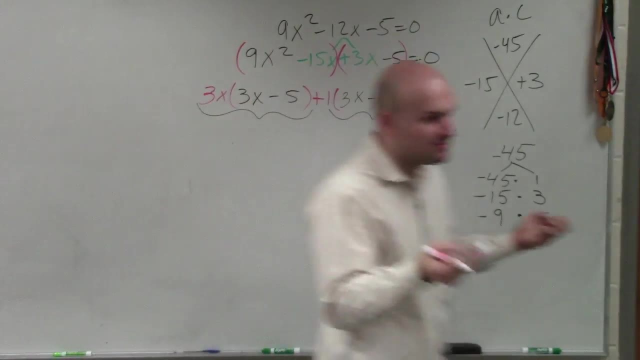 Now what you guys can see is that the 3x minus 5 is common between both of these terms or both of these expressions, Right, Do you guys see? I have two expressions that are separated by addition And therefore now you factor those out. 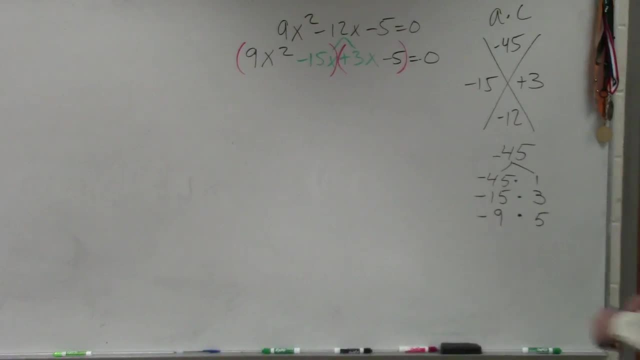 but we also talked about factoring out the GCF. Now, all you're simply going to do is factor the GCF out of each of these expressions. So we look at the first two and say: what do these have in common? What is my common factor? 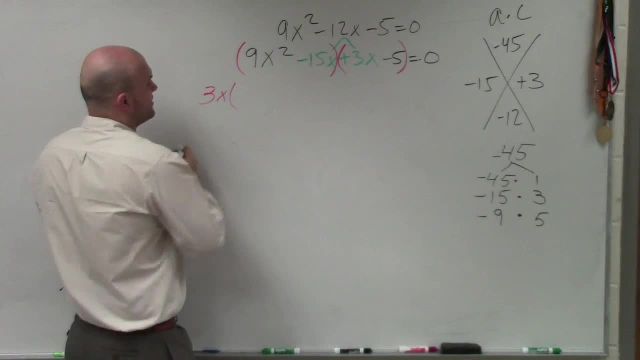 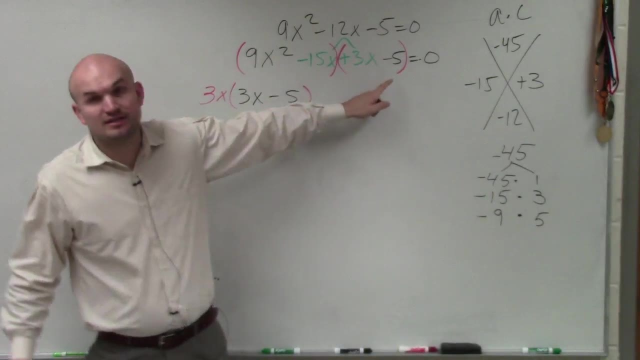 You could say a 3x, And when you factor out a 3x, you're left with 3x minus 5.. Then I look over here and I say, is there anything I can factor out of these? No, So therefore I can factor out a positive 1..